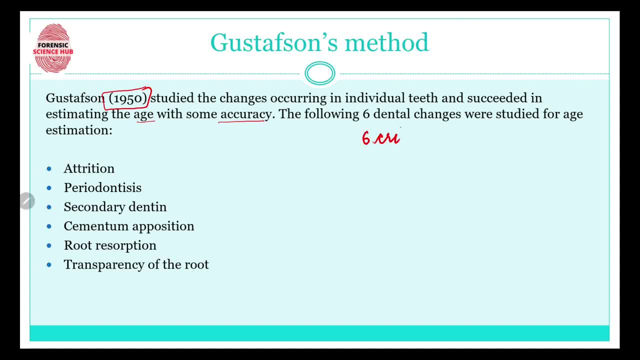 teeth. He proposed six criterias on the changes that occurs in the teeth with age and he developed a ranking scale. A ranking scale was developed by him. The scale goes from 0 to 3, that is, 0,, 1,, 2 and 3.. And the six criterias that he used are attrition, periodontosis, secondary dentine, cementum, apposition and transparency of the root. All these six criterias were studied for age estimation. So in the year 1950, Gustafsson came up with a method for calculating the age of a person on the basis of six criterias. All these six criterias were studied for age estimation. So in the year 1950, Gustafsson came up with a method for estimating the age of a person using the root. All these six criterias were studied for age estimation. So in the year 1950, Gustafsson came up with a method for estimating the age of a person using the root. All these six criterias were studied for age estimation. So in the year 1950, Gustafsson came up with a method for 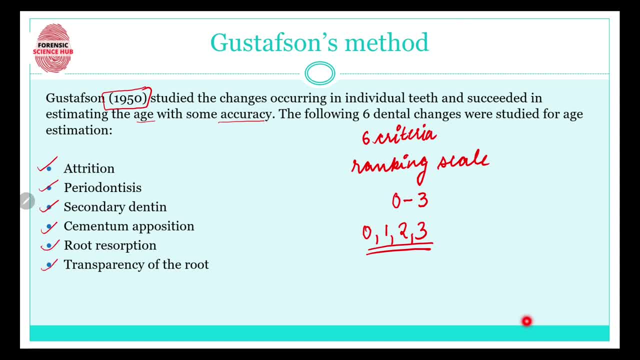 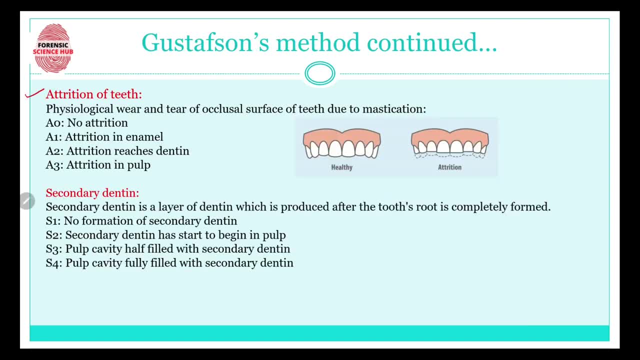 epization, root resorption and transparency of root. now let's study these six criterias one by one. first is attrition of teeth. what is attrition? attrition means physiological wear and tear of occlusal surfaces of the teeth due to mastication. now our teeth are responsible for a number of 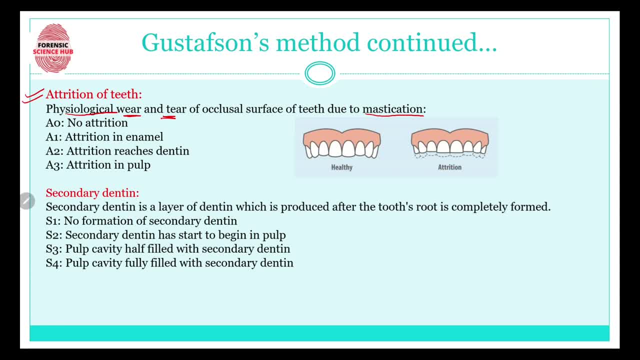 reasons like grinding, chewing, tearing, etc. right. so with time, what happens is that the wear and tear of teeth starts to occur, due to which attrition occurs. this, you can see over here, is a healthy teeth, whereas this is a teeth in which attrition has occurred. the teeth were 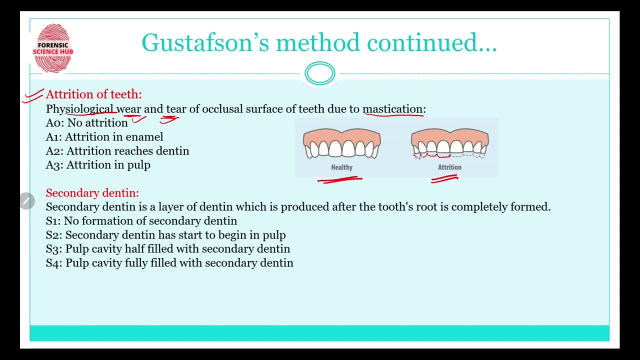 supposed to be till here, right as you can see, but due to its wear and tear it has decreased in its length. so we have four scales for attrition, that is, a 0, a 1, a 2 and a 3. as i said in this method, the six. 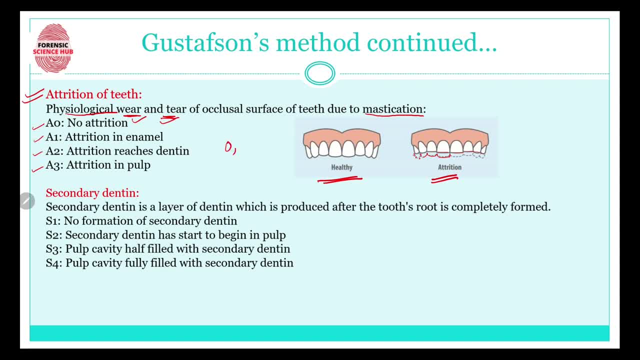 criterias have been ranked on a scale of 0, 1, 2 and 3, so here we have a 0. a is because we are studying the criteria of attrition, so a is used. a 0 means there is no attrition. a 1 means that attrition is. 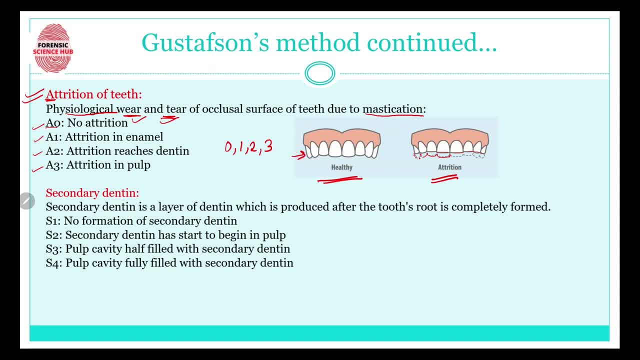 antigenically 걱정 headphones. Generation A and B: more aggressive people. In the 2500 studies we area A2 means attrition has reached the dentine A3. most severe one means that attrition has reached the pulp area. Then the second criteria is secondary dentine. Secondary dentine is a. 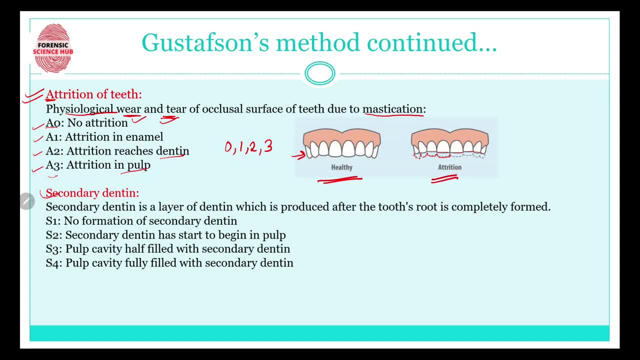 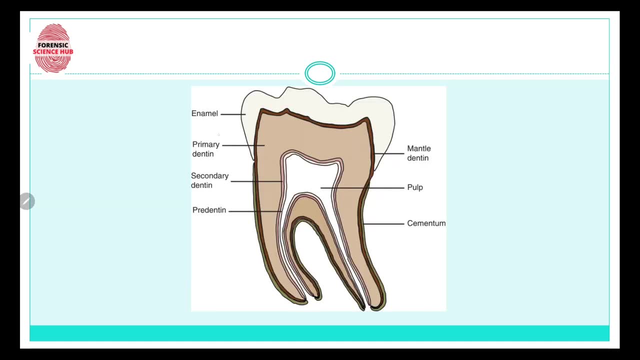 layer of dentine which is produced after the tooth's root is completely formed, So with age. so normally we have only one dentine, but with age what happens is a secondary dentine starts to get formed. Here you can see in this picture: this is the. this area is the primary dentine area. 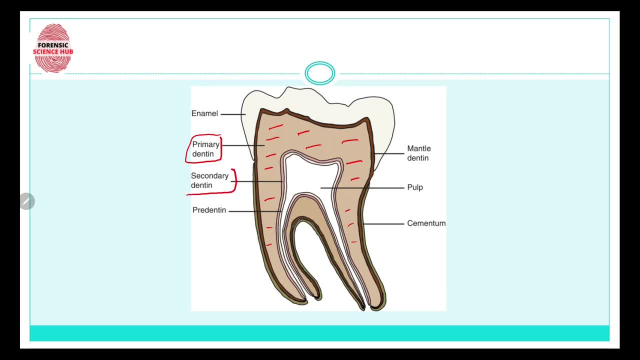 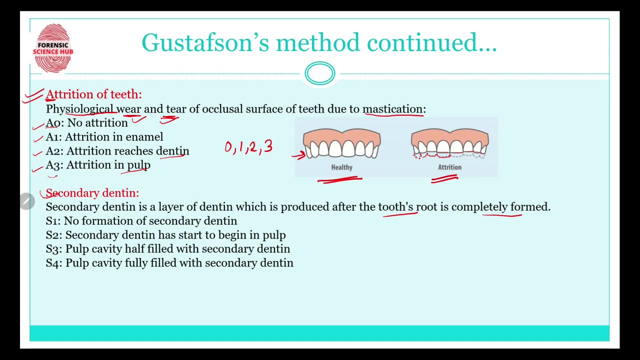 but with age what happens is we get to see a secondary dentine area also. So this area here you can see this is the secondary dentine area. all right, So the four scales are s. there is a mistake here. this has to be s0, s1, s2 and s3. okay, s0 means that there is no formation. 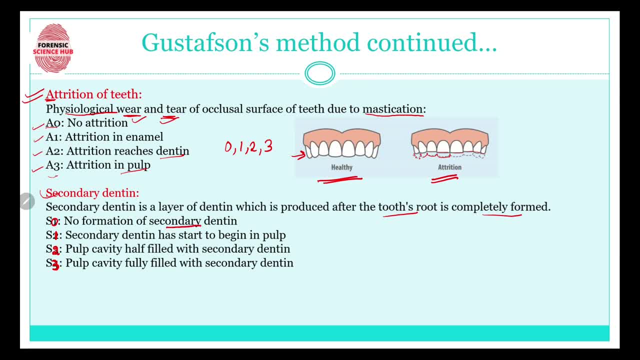 of secondary dentine. s1 means the secondary dentine has start to begin in the pulp area. s2 means pulp cavity has half filled with secondary dentine. s3 means pulp cavity cavity is full filled with secondary dentine. so these are the four scales of secondary dentine criteria. 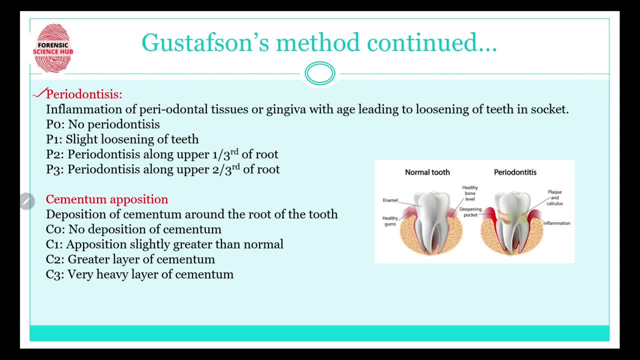 now let's talk about the third criteria, that is, periodontosis. periodontosis basically is the inflammation of periodontal tissues or periodontal ligaments or gingiva with age that is leading to loosening of the teeth in the socket. so basically, in periodontosis, the gingiva, the gums or the 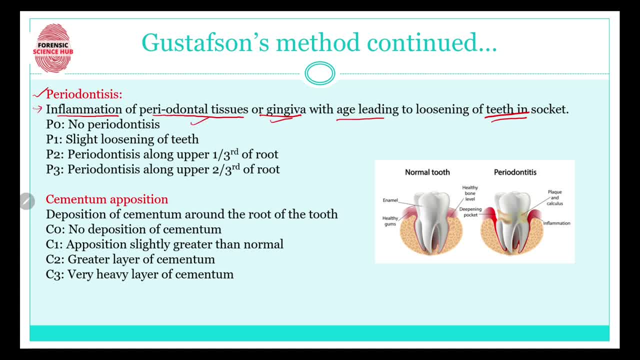 periodontal ligaments are the ones that are the most affected by periodontal disease. so these gums is, they are getting inflamed, got to which what happens is that the teeth start to become loosened in the socket. there's no probably grip here. you can see in this: 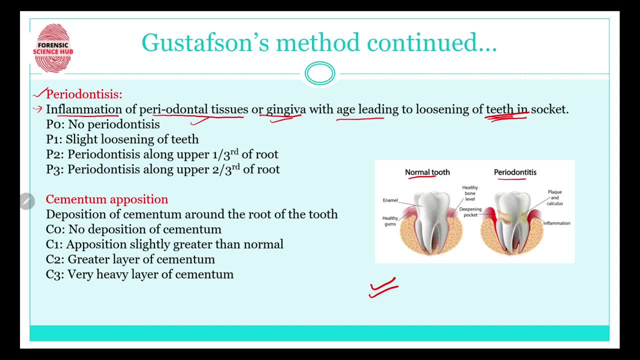 picture. this is a normal tooth and this is a tooth having periodontosis. here we have this red area that you can see. this is gum area, alright, and here we have the heaway gums. but in case of periodontist, i will talk about if you do not go. so this is gums, so bollywood. gums. European gum jones jones jones. gum jones gones, acetone that can be practiced in gums. almost all the gums probably gets stomach cancer. gum jones gones gones, meaning gum healings, but the gums will increase this more and this also health and health and, in my opinion, periodontal. 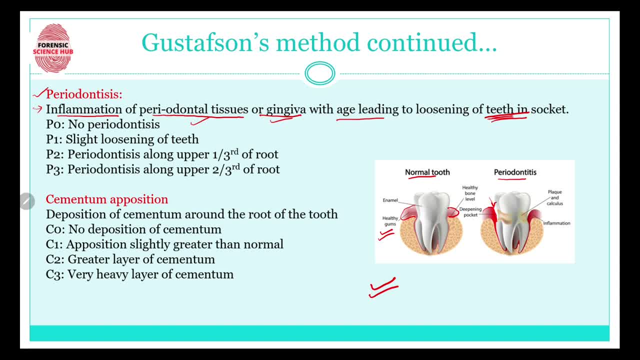 displaced from its normal position. there's a gap that you can see over here. this gap is due to the inflammation of gingiva or the periodontal ligament. so this is what happens in periodontosis. here we have four scales: p0, p1, p2 and p3. p0 means there's no periodontosis, p1 means that slight 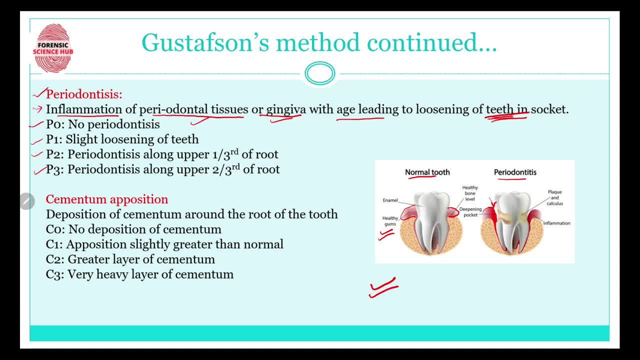 loosening of teeth has started. p2 means periodontosis along one third of the root has started and p3 means periodontosis along upper two third of the root has happened. so, basically, how are we going to use this method? we are going to see the teeth of the person. we 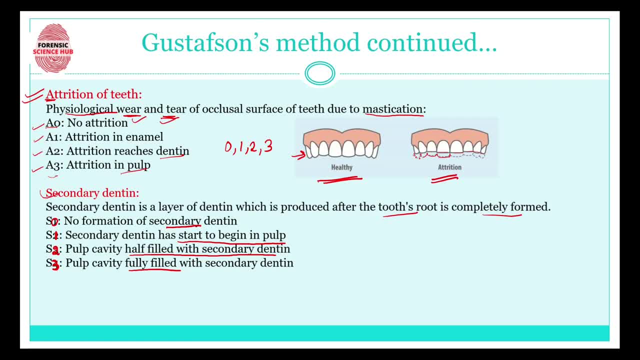 are going to see how much attrition has occurred. has the attrition just reached the animal or has it even reached the pulp? if it has reached the pulp, then we are going to see the teeth of the, the person to have the score of a equals to three. then we'll look for dentine has. is there any? 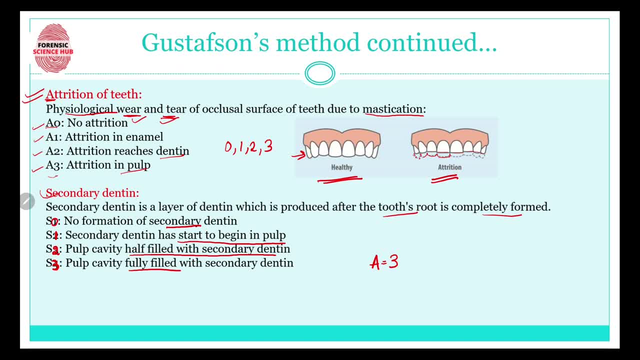 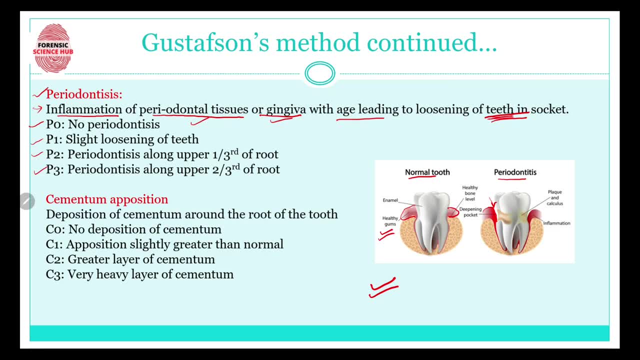 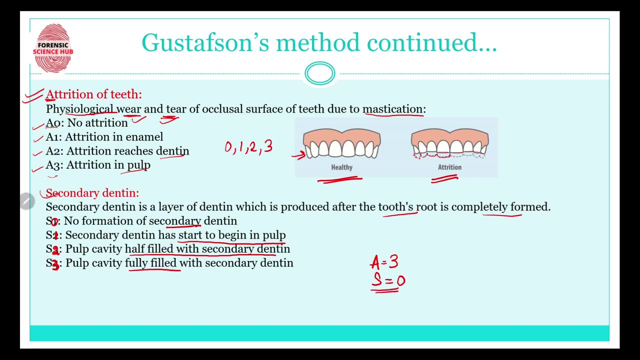 dentine formation is a secondary dentine formation. no, there is no. if there is no, then s value will be zero and later on we are going to calculate for all of these criterias. we're going to calculate and then we have a formula at the end, on the basis of which we are going to calculate the entire age. 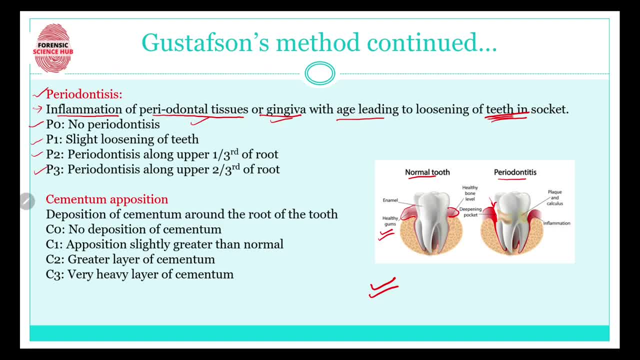 of the person. all right. so coming back to the fourth um uh criteria, that is, the cementum apposition, that is, that means the deposition of cementum around the root of the tooth. so c0 means that there is no deposition of cementum. c1 means apposition is slightly greater than normal. c2: 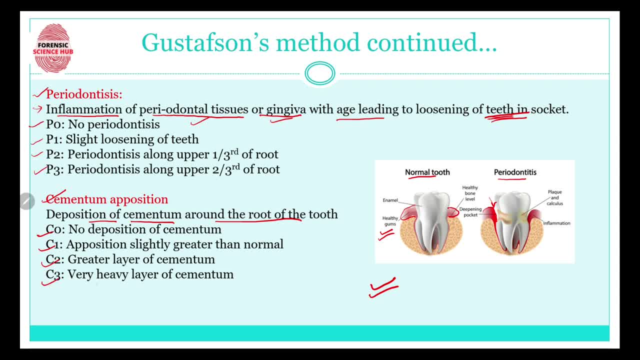 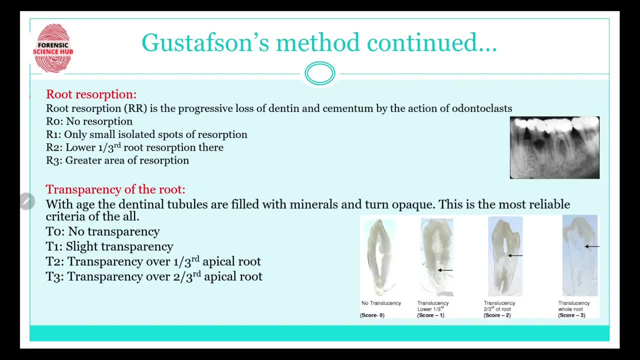 means there is greater layer of cementum and c3 means there is very heavy layer of cementum. all right then next criteria. fifth criteria is the root resorption. root resorption is the progressive loss of dentine and cementum by the action of odontoclast cells. so we know that there are two types of cells that 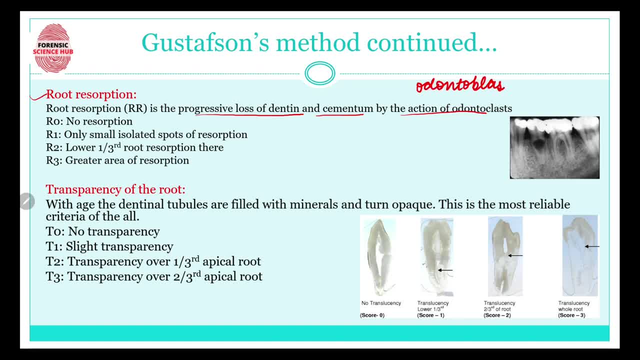 is odontoblast cells and odontoclast cells. odontoblast cells are responsible for the formation of tooth cells- okay- whereas odontoclast cells lead to degradation of the dental cells. odontoclast cells are basically responsible for the resorption of the root of the deciduous teeth. so root resorption basically means that there is 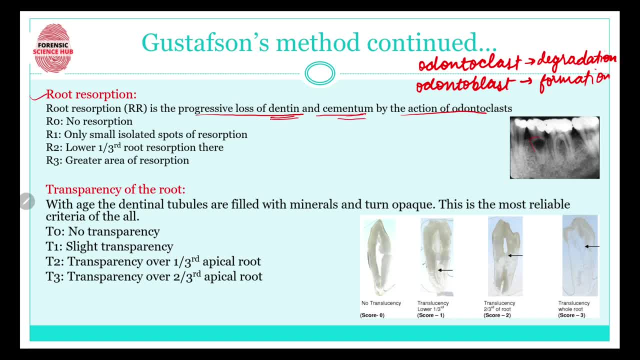 loss of dentine and cementum. here you can see in this area the root, in this um radiograph over this area you can see that the root resorption has been shown. so r0 means there's no root resorption. r1: only small, isolated spots of resorption can be seen. r3- r2 means lower. one third root resorption is. 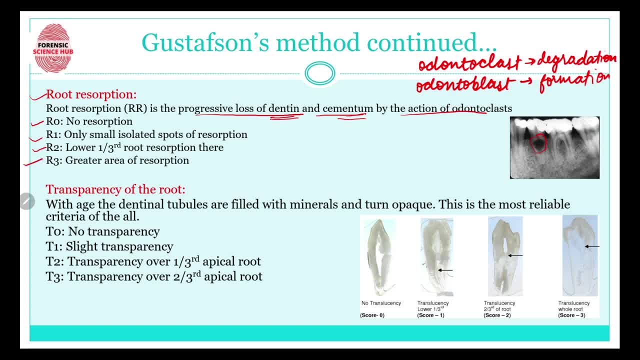 there, and r3 means that there is greater area of root resorption then um. the last criteria is the transparency of root. with age, the dental tubules are filled with minerals and they start to turn opaque, due to which the root starts to become a slight transparent. this is the most reliable. criteria of the all this is zero. R2,, R3,, R3,, R3,, R3, R3 and R3 is the most reliable criteria of the all this is zero: R1,, R3,, R2,, R3 and R3.. 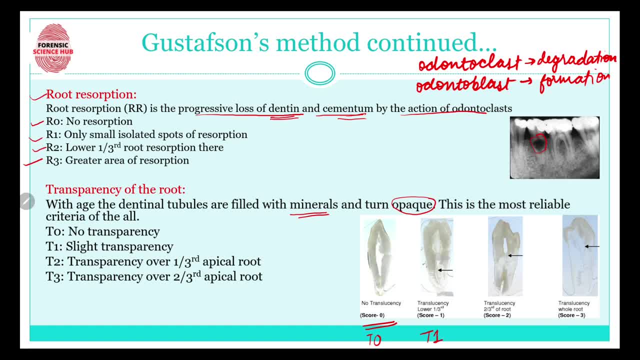 that is t0 score. then here comes t1 score, that there is slight transparency. then here we have t2, which means transparency is over one third of the apical root, and t3 means the transparency is over two by third apical root, which will also include transparency in the whole root. so these 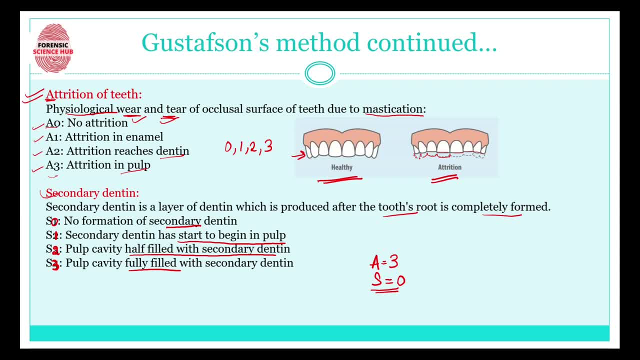 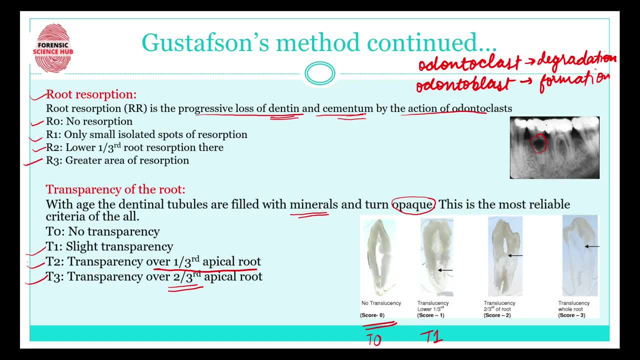 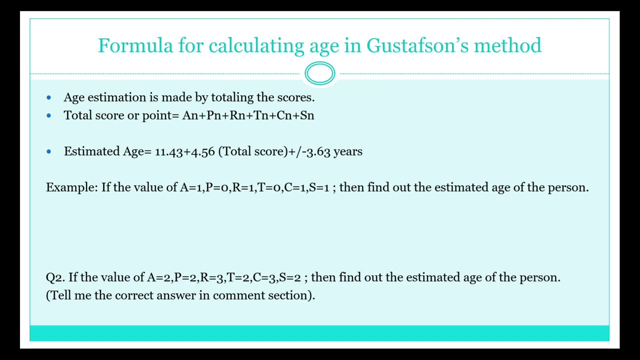 are the six criteria, that is, that are used in the gustafsans method: attrition, secondary din time, periodontosis, cementum apposition, root resorption and transparency of the root. now let's see the formula that is used for calculating the age in gustafsans method, so the age estimation can be. 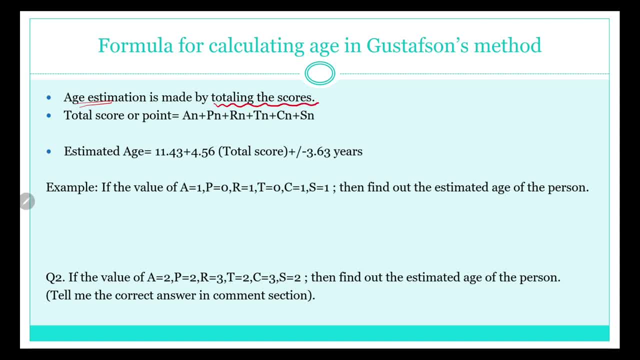 done by totaling the scores: total score. how we are going to calculate a score plus p, score plus r, score plus t, score plus c, score plus n score, that is, attrition score, periodontal score, root resorption score, transparency of root score, cementum, apposition score and secondary dentine. 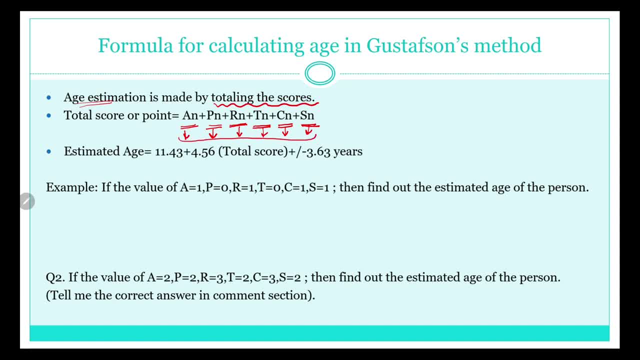 score. all right, these scores has to be added up and these this score is to be kept over here in this formula that is, in the total score area. so basically, the formula that is used is 11.43 plus 4.56 into the total score that we will be getting from here after the proper examination. 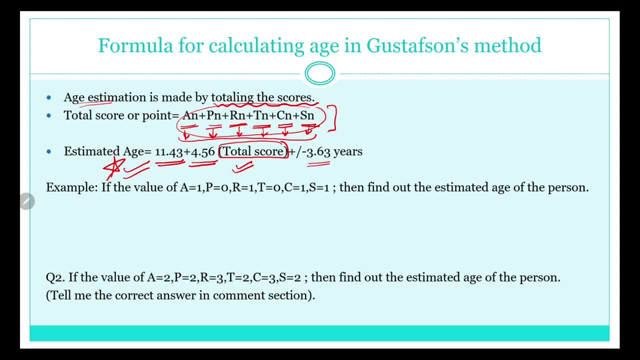 of the tooth, plus minus 3.63 years. so let's try to find out with the help of an example. if we have studied a teeth, then we are going to have all these values of a and for p, for r, for t, for c and for n. we'll be having these values, right. what does the value? 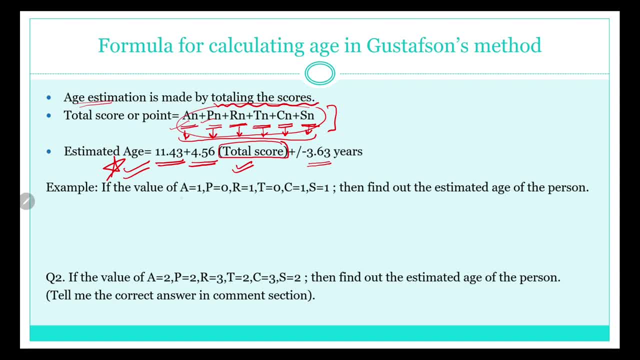 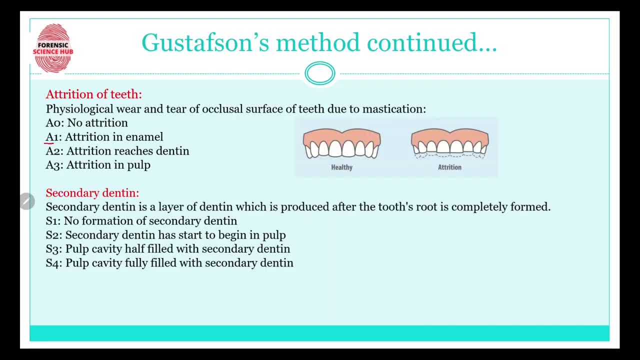 means like um. in this question we have the values: a equals to one. what does a equals to one means? a equals to one means that attrition is in the animal. so we studied the teeth and we found out that attrition has only reached the animal portion. so we deduce that a equals to one. similarly, we 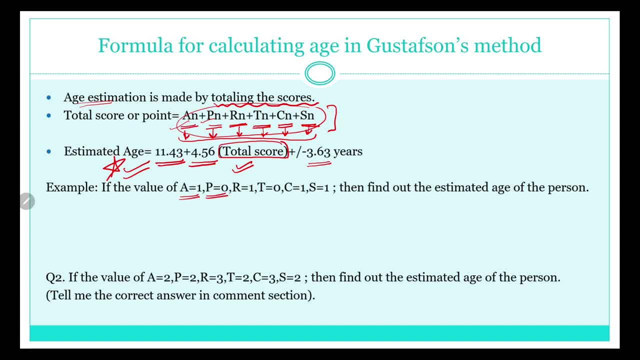 have here: p equals to zero. p equals to zero. that means that there's no periodontosis, no inflammation, right? so, accordingly, we have been given these values, but we just have the values. how can we calculate the age of the person? so we'll be doing that with the help of this formula. remember this. 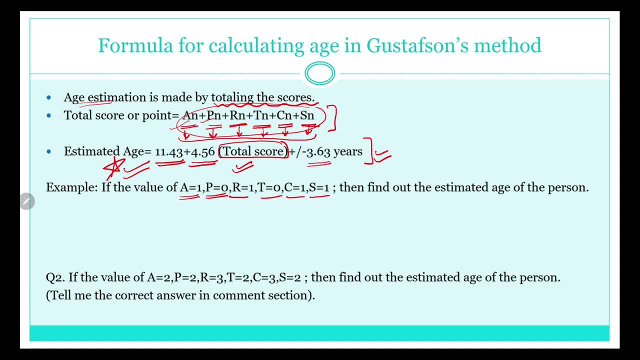 formula. so if these values are given, so let's find out the um age of the person, which is going to be 11.43 plus 4.56 into the total score, what will be the total score? total score will be 1 plus 0 plus 1 plus 0 plus 1 plus 1 right. 1 plus 0. 1 plus 0 plus 1 plus 1 right.